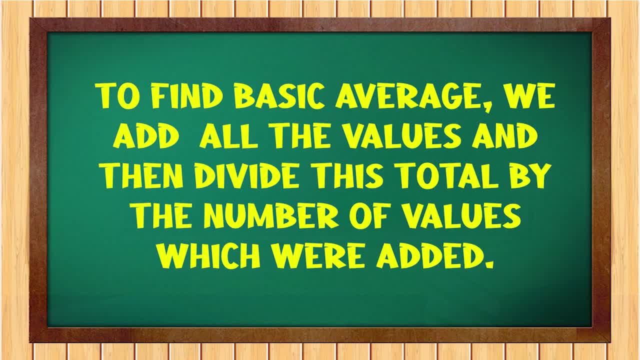 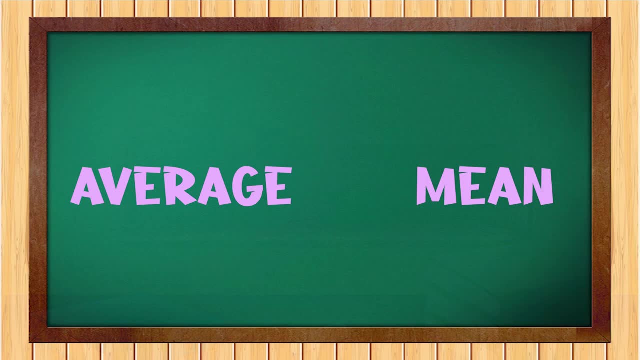 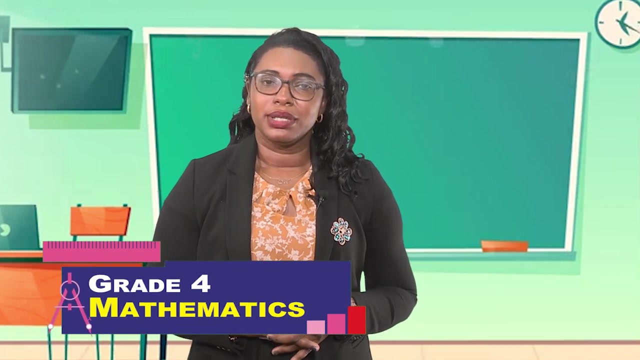 To find basic average, we add all the values and then divide this total by the number of values which we added together. We also discussed that we can use the term average or mean, because they mean the same thing. At the end of our last lesson, I also gave you homework. Did you complete that? 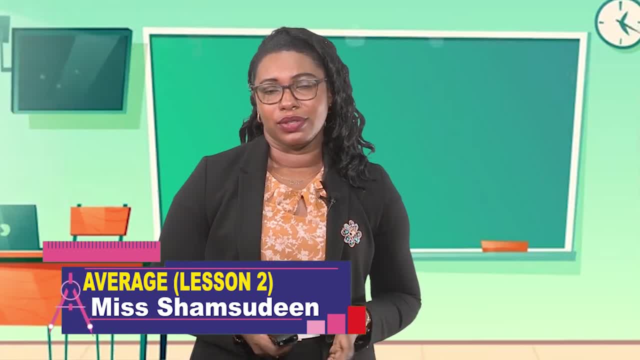 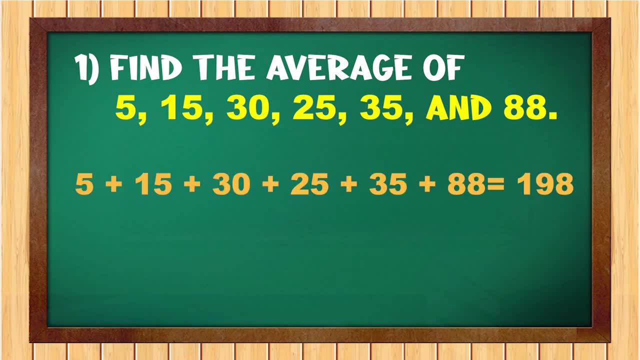 If you did. let's quickly look at how you solve them. Number one: you had to find the average of a set of numbers I gave you. If you did that one and you added correctly, you should have gotten a total of 198.. Now, because you added six different numbers, you had to divide 198 by six. If you did, 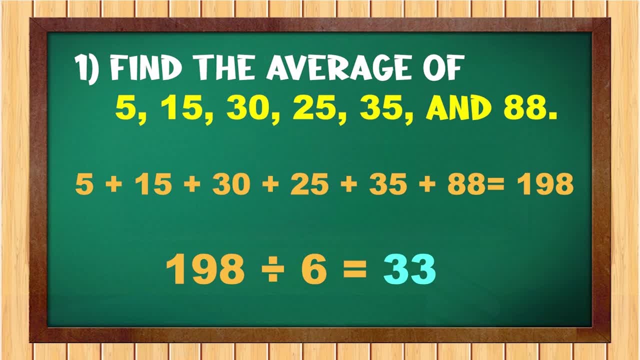 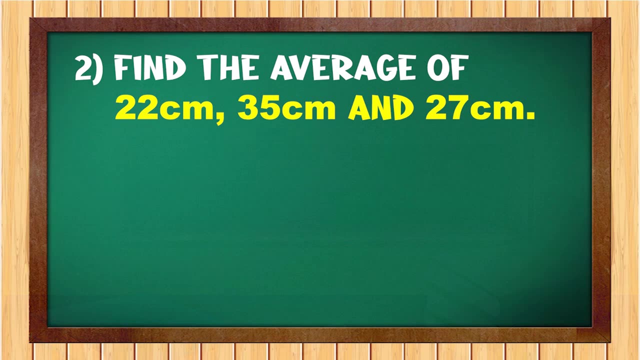 it correctly, your answer should be 33.. So the average or the mean of those six numbers is 33.. For number two, you were given three sets of numbers. You had 22 cm, 35 cm and 27 cm. Again, if you added these numbers correctly, you should have gotten 84. Now, 84 should have been. 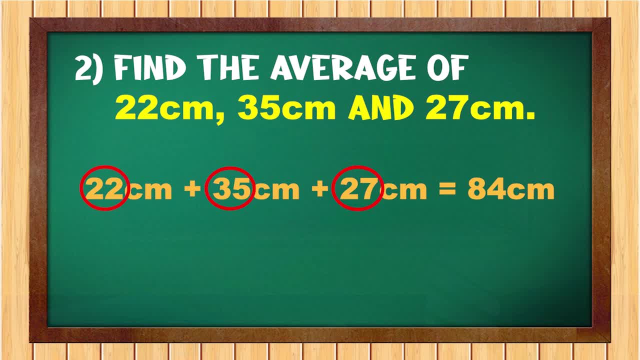 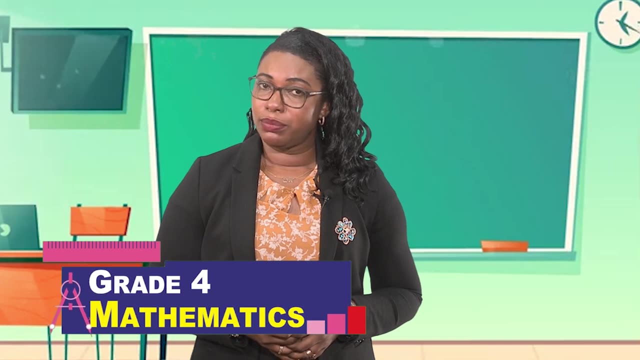 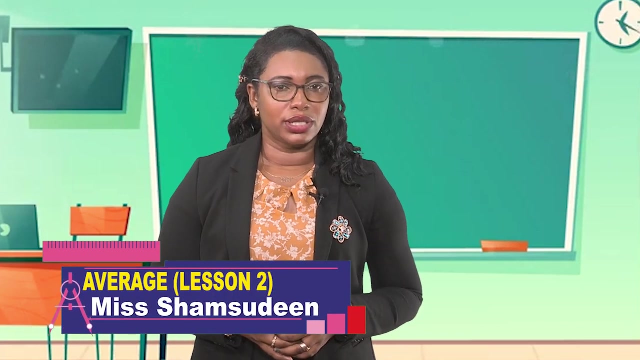 divided by three, because you added three sets of numbers. If you divided correctly, your answer would be 28.. So the average of those three sets of numbers will be 28.. Did you get both for the homework correct? Well, I hope you did. For today's lesson, we will concentrate on finding missing. 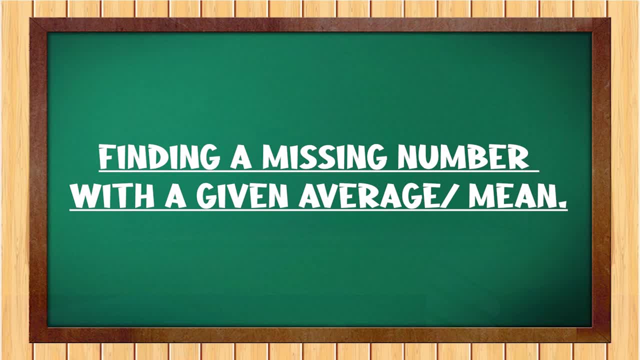 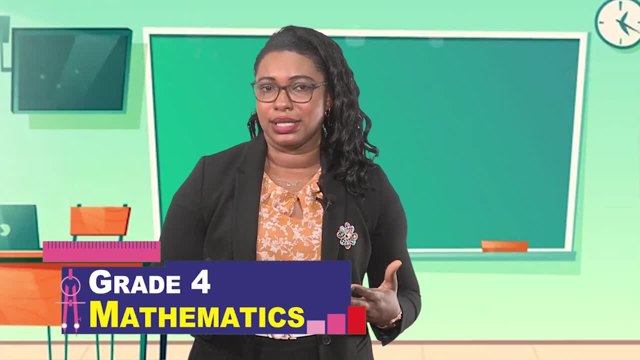 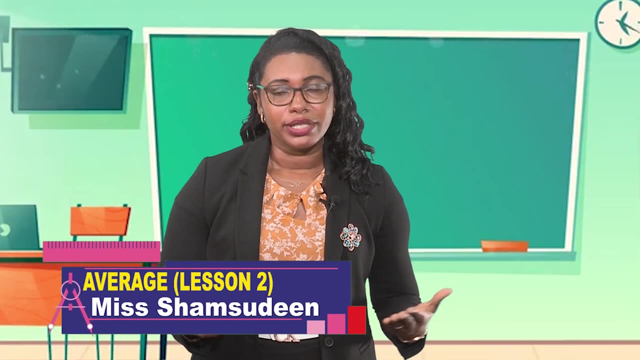 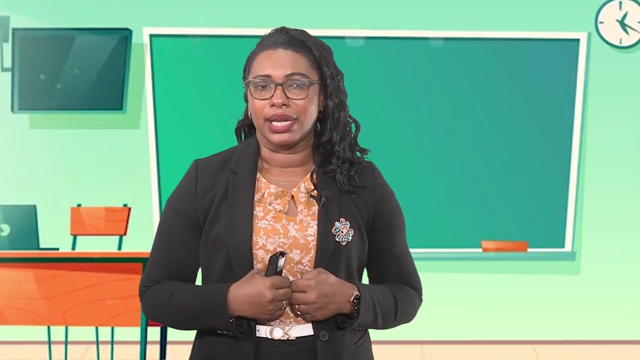 number with a given average or mean. What it means is that you were given what the average is or the mean what it is, and then you have to find what was one of the quantities that was added with another set of quantities to give you a particular average. Now how do we go about doing that? Let's look at these. 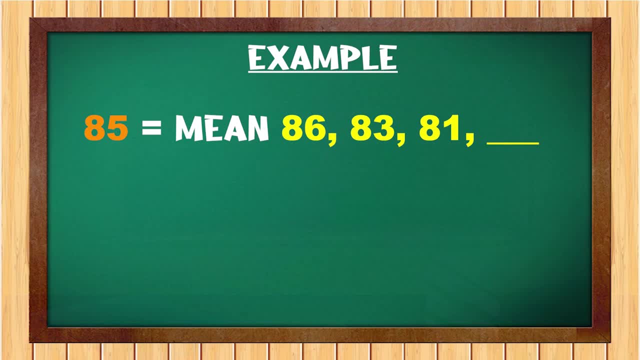 examples. Now you're given the mean 85 and you're given 3 out of 4 numbers. We have 86,, 83 and 81. You have to find the fourth number that would give you an average of 85. Now what do you do? 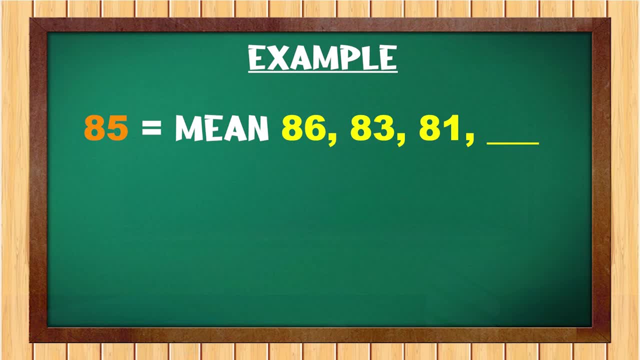 Because in this case you have four numbers that will give you the mean of 85, you simply multiply 85 by 4 to get the total needed. So if we multiply 85 by 4, you should get a total of 85.. 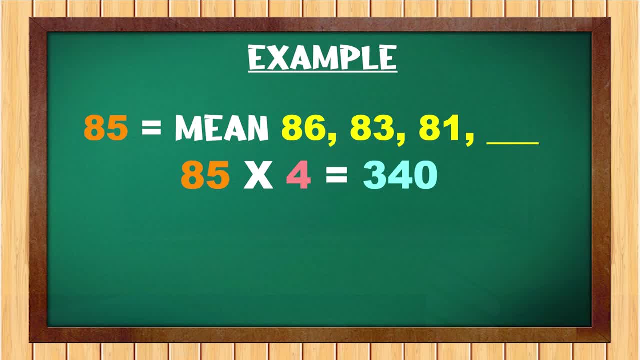 So we get 340.. That's the average being multiplied by the amount of values that was added or should be added. to give you that average, We then take the three known values, which are 86,, 83 and 81, and we add them together. So we know these three numbers because we see them. We add them together. 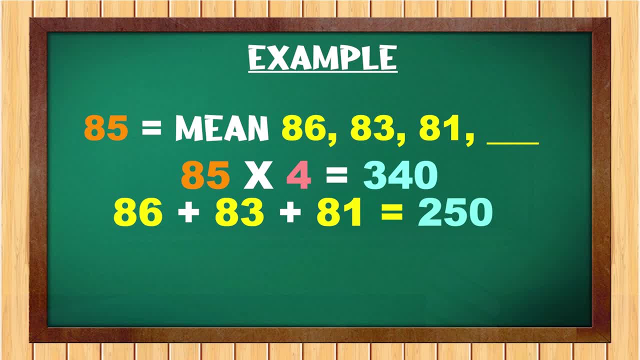 We have 86 plus 83.. Plus 81,, we will get 250.. Now that we have two sets of sums or totals, we do subtraction. Remember we always take the smaller number from the larger number- And so what we should have now. 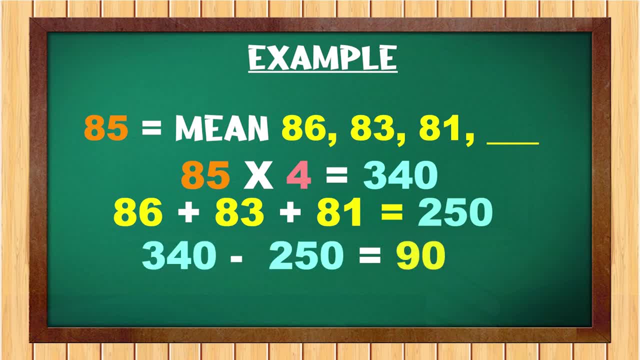 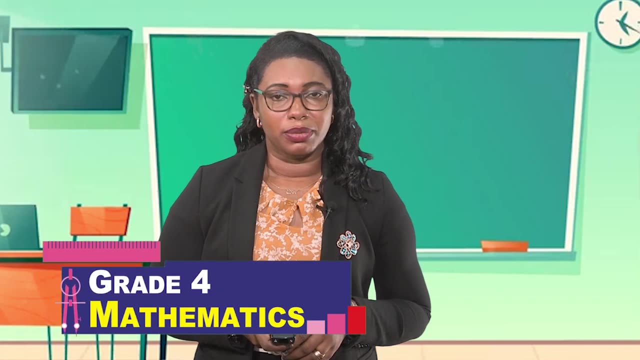 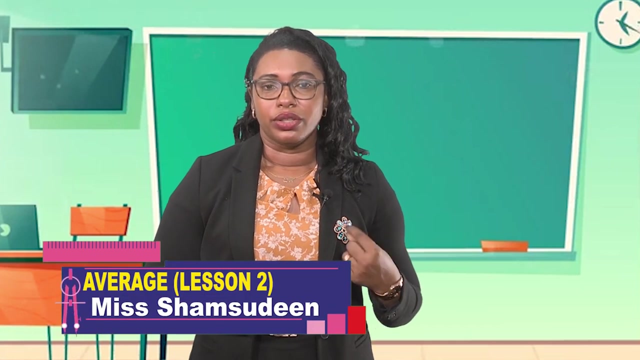 is 340 minus 250, which would give us 90. So in this case, 90 will be the missing number. Make sure that you look at how these problems are set down, how you write your digits under digits, each value under the correct place, so that your answer, after you're working out, will be: correct. So let's look at that again. You first multiply the mean by the amount of values that were indicated. You multiply the mean by the amount of values that were indicated. So you multiply the mean by the amount of values that were indicated. 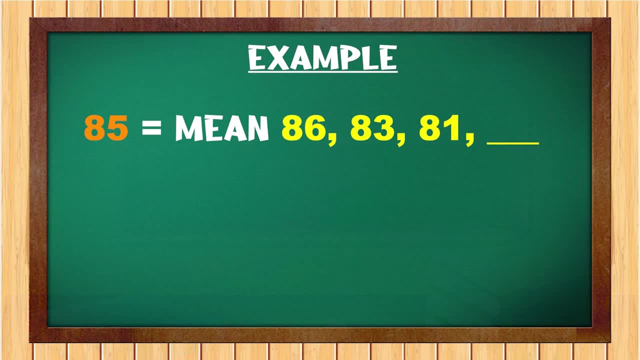 You multiply the mean by the amount of values that were indicated. So you multiply the mean by the amount of values that were indicated. So we know we're supposed to have four sets of numbers. We multiply 85 by four And then we add the three known values, which are 86, 83 and 81.. 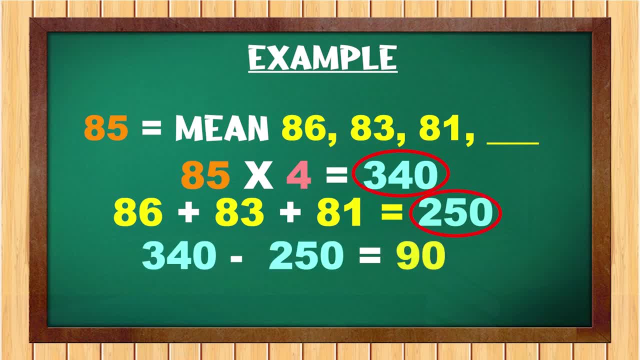 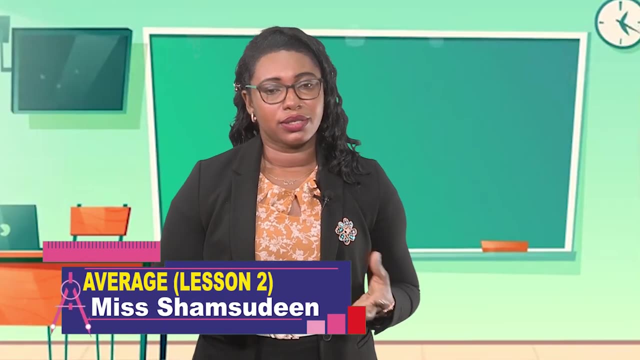 We then do subtraction with the two totals that we would have got from those two separate operation. When we do that, we get 90, which represents the missing value. Now, if you want to verify whether or not this is correct, you can simply follow the steps we did in our first lesson. 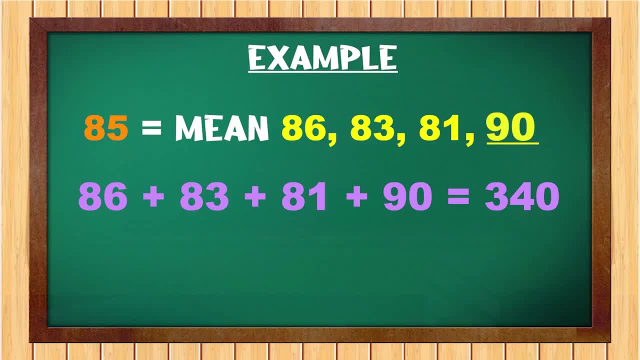 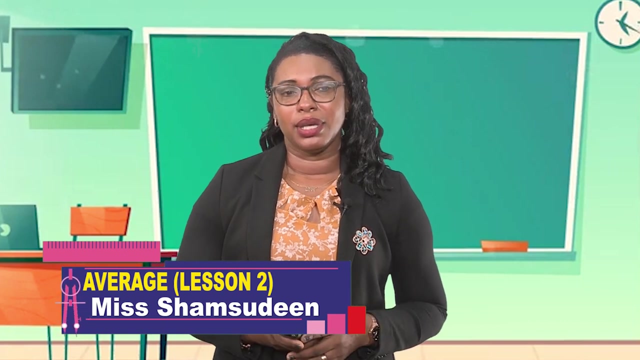 on average. and now you could add 86, 83, 81 and 90 and then divide it by 4 to see if you will get 85.. once you get 85, you will know that your answer is absolutely correct. now let's look at this example, this time in awarded form. Mr Banks sold newspapers for five days. 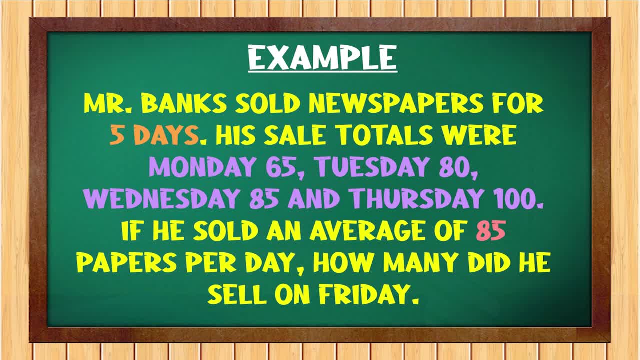 his sale totals were: Monday 65, Tuesday 80, Wednesday 85 and Thursday 100. if he sold an average of 85 papers per day, how many did he sell on Friday? now you could add mach, some winners, some answers, and then divide by 4 to see if you will get 85. 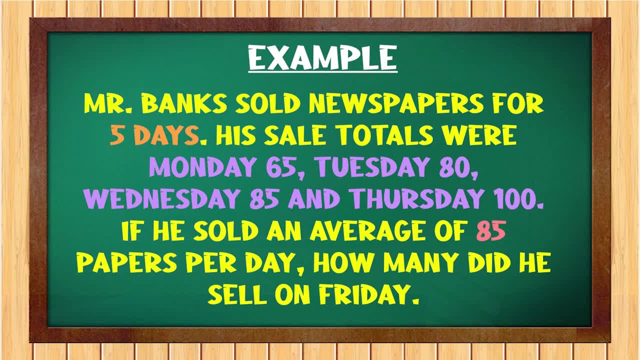 Now for this problem. we use all the information that has been provided in order to solve what was asked. So what do we know? We know that he sold papers for five days. We also know that over the five days, he sold an average of 85 papers per day. 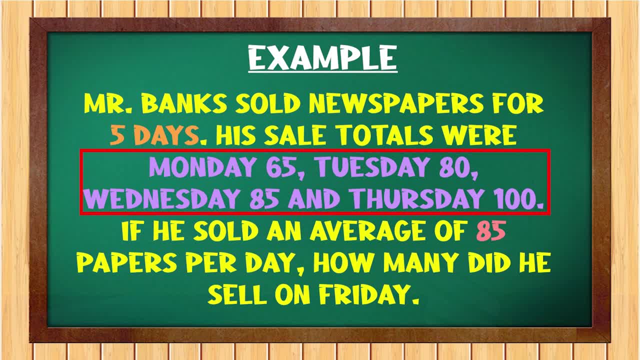 And we were given the total sold for four days. What is it that we have to find out? We are asked to find what was the direct amount sold on Friday, which was the fifth day of his sales, But we also need to figure out what was the total of papers sold over the five days. 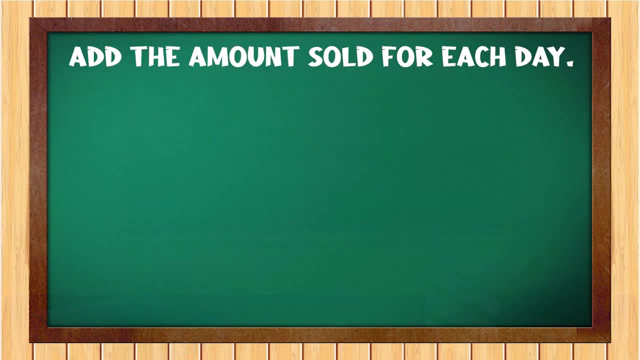 So how do we go about doing that? Again, we add the amount sold for each day, And that would give us Monday 65 plus Tuesday 80.. Wednesday 85 and Thursday 100.. We will end up with a total of 330. 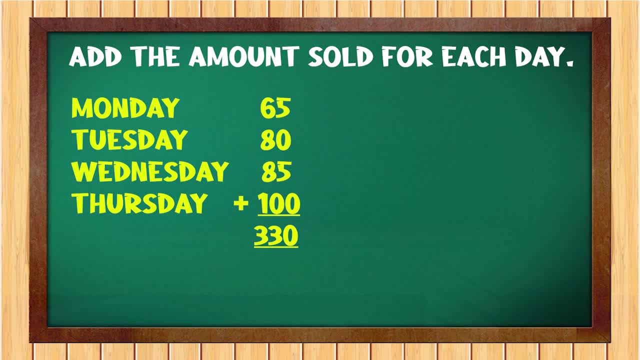 So we know, for the four days we sold 330 papers. Then remember it said that 85 was the average sold over the five days period. So which means that we will now multiply 85 by 5.. Now some persons who get a little challenged with that: 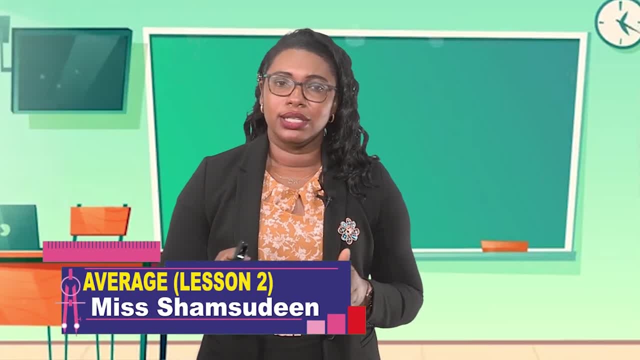 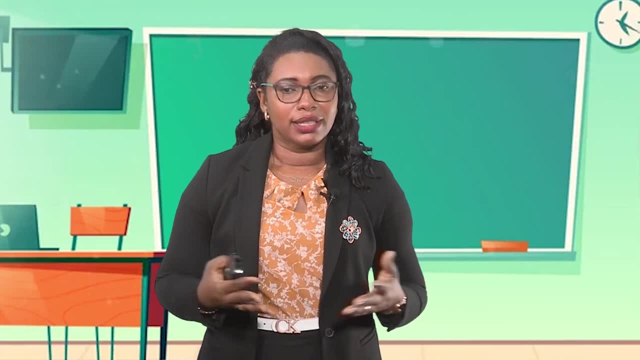 Let's see what the answer to this question is. We're saying the average is: each day he sold 85. So if you want to add 85 five times, which might take a little time, You should get the same answer as if you were to multiply 85 by 5.. 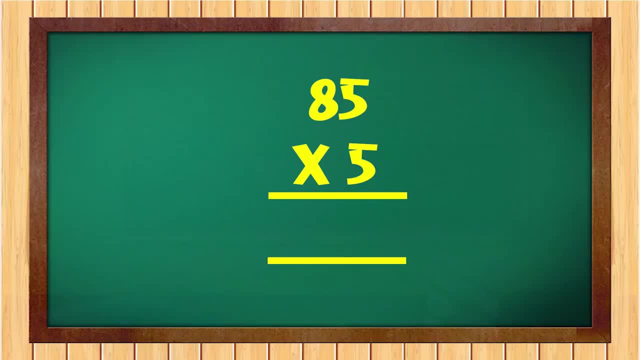 Now again, we set down 85 multiplied by 5. You will get: 5 x 5 is 25.. And we will take that 5 from the 25 and we will write it on our answer line five. it's 40. and then we add that two from the 25, we get 42. so our answer there is 425. 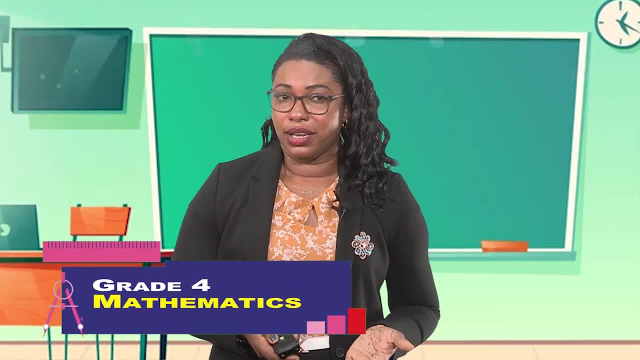 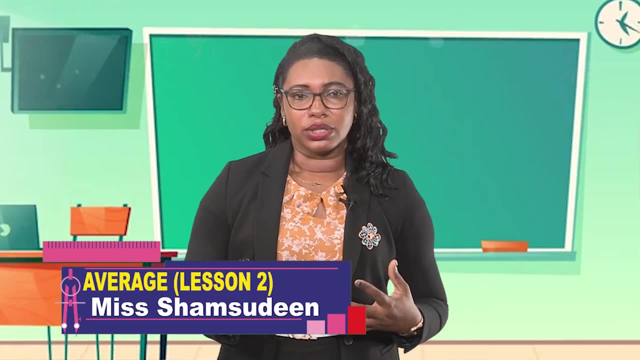 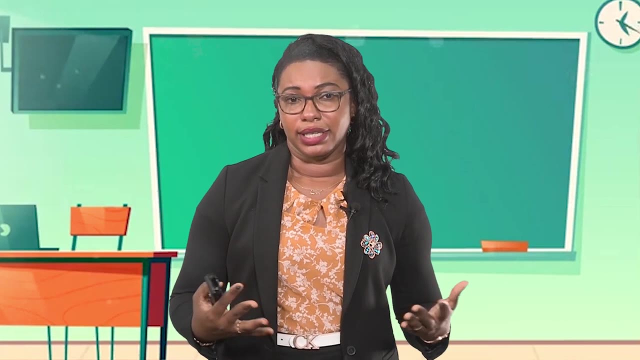 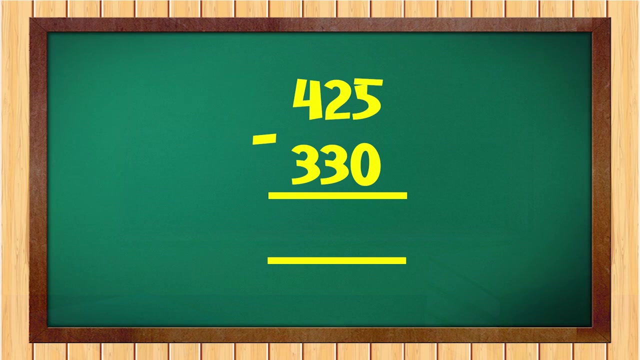 so how do we find for the friday value? well, we now have to subtract. so we use the two amounts and we subtract because we do not know the exact amount sold on friday. so here we have 425 minus 330. when we do that, we find the difference between the two amounts. 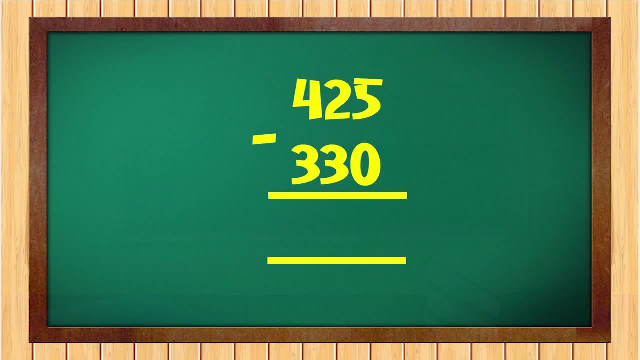 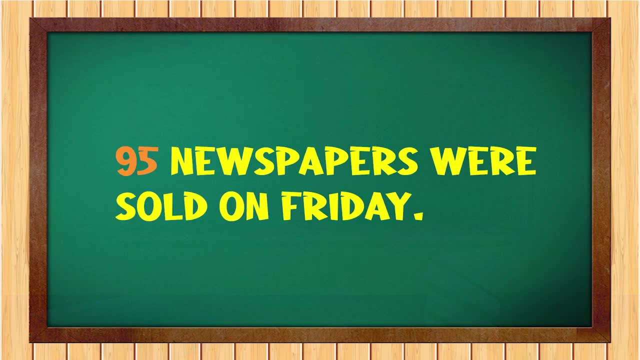 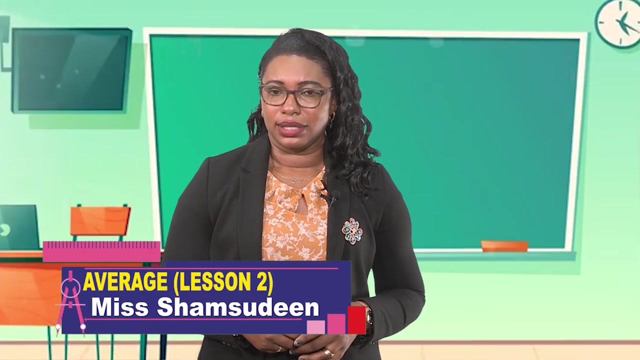 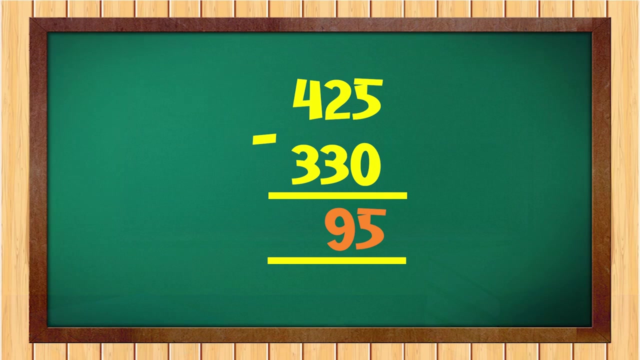 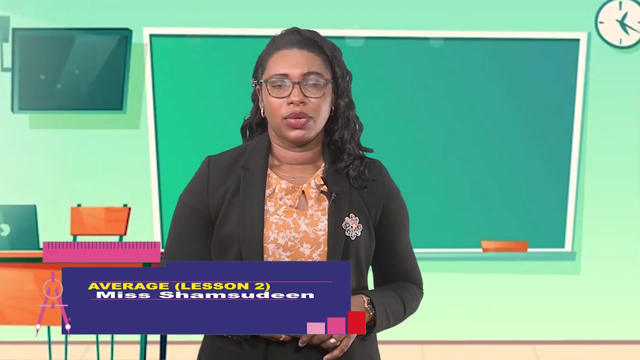 which represents the exact amount sold on friday. our answer will be 95. so 95 newspapers were sold on friday. let's take a few seconds and look at that operation again: 425 minus 330, remember, digit under digit and in the correct place value. now we can verify to see if our 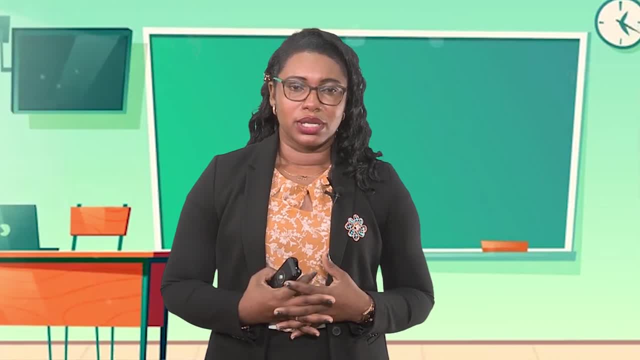 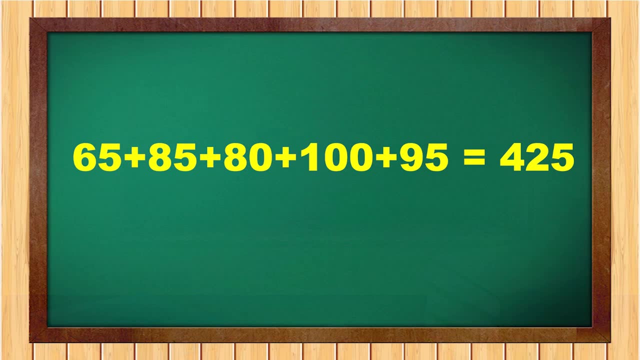 answer is correct again by adding those amounts- the 65, 85, 80, 100 and the 95 that we just figured out for Friday. we add them together to see if we would have gotten 425, just as we multiplied the 85 times 5.. Once we get that divide, 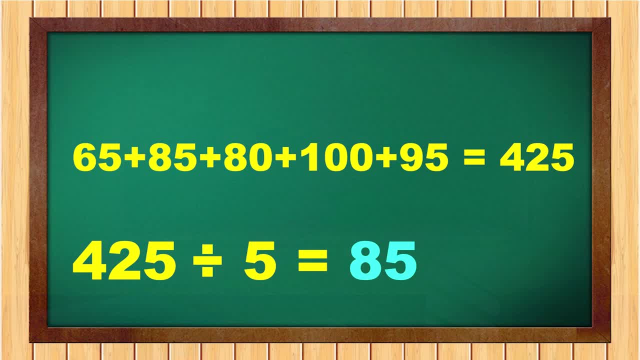 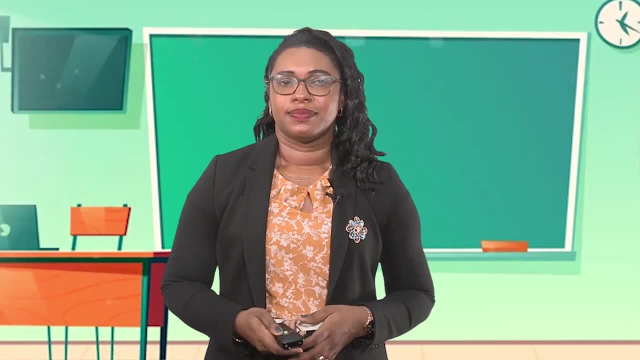 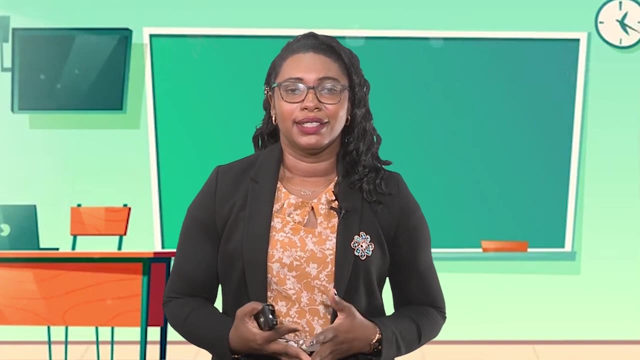 that now by 5 and see if we will end up with 85. If we do, we will realize that our answer is absolutely correct. Now I hope you have your pencil and your books and you are ready to try to find these on your own. The first one I'm giving you: 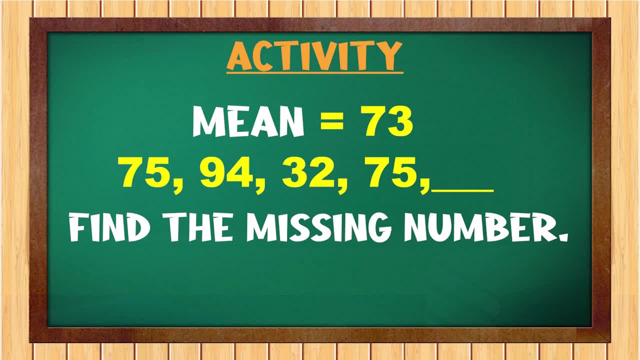 the mean. Remember it's the same as the word average. I'm giving you the mean 73.. I'm also giving you the numbers 75,, 94,, 32 and 75.. You have to find what is the fifth number. I'm giving you 60 seconds to go ahead. 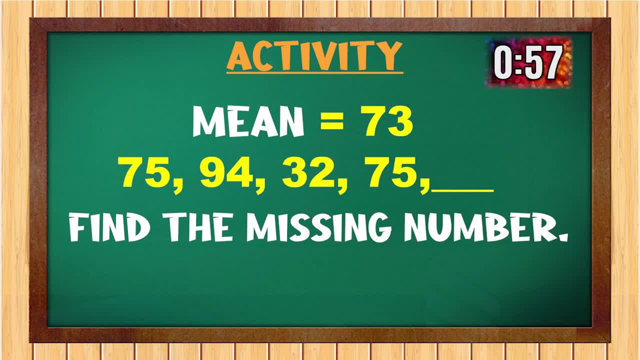 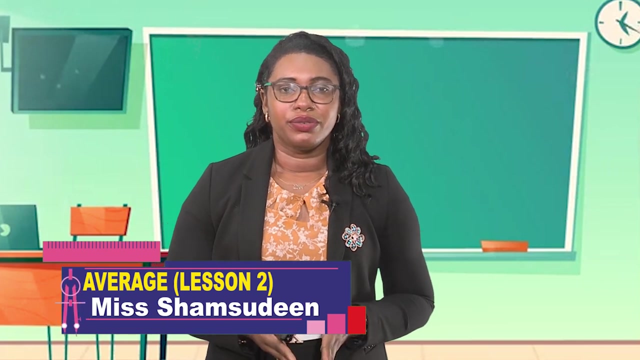 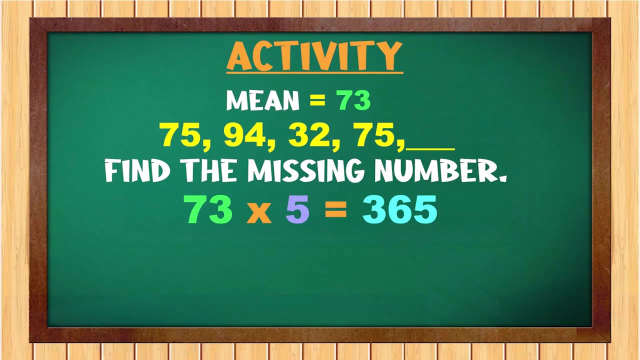 and find it, and find that, and find that and find are burn the, the. now let's see how well you did. 73 was the mean given for the five numbers of which you were given for. so you multiply the 73 by 5, which would give you a total of 365 once you would. 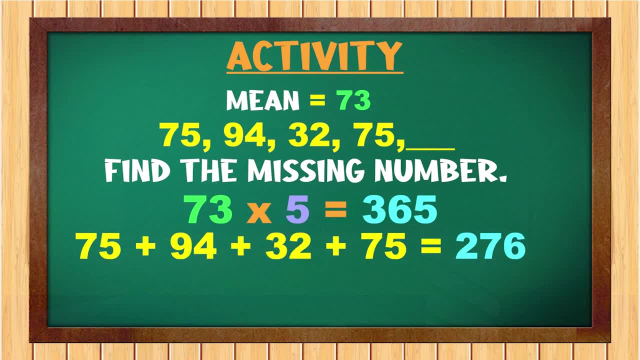 have added correctly the numbers that you know, which were given to you. the four numbers in total will give you 276. now that you have the two totals, 365 and 276, it's time for you to do your subtraction. so 365 minus 276 should give you 89. 89 would represent the number that is missing. 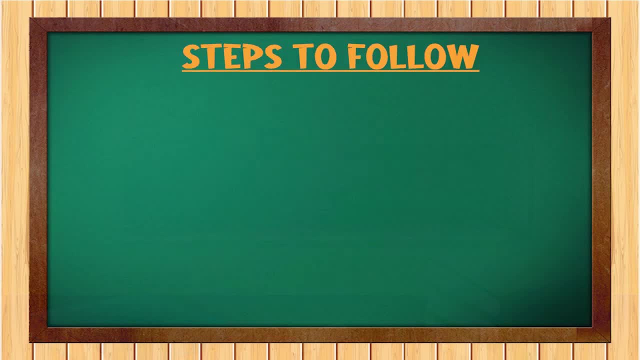 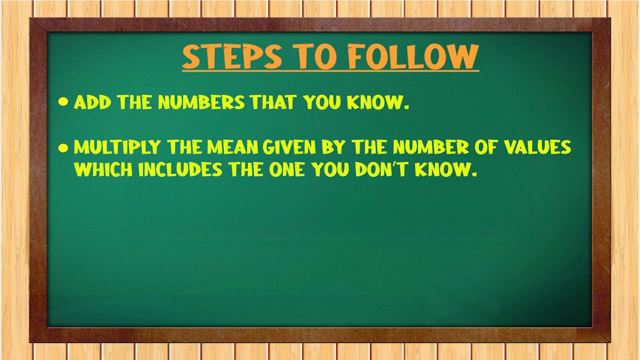 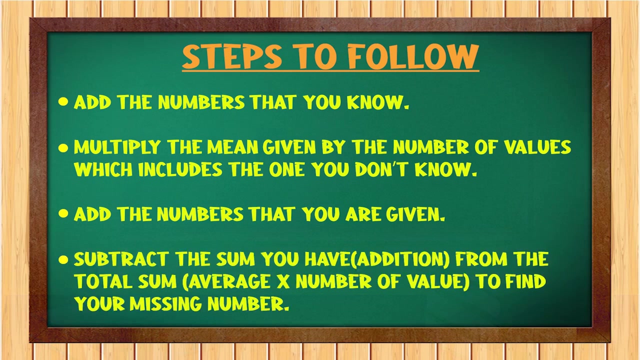 so let's look at the steps that you would have followed. first, you added the numbers that you know. you multiplied the mean that you were given by the number of values, which includes the one you don't know. then you added the numbers that you were given. you subtracted the sum you have from. 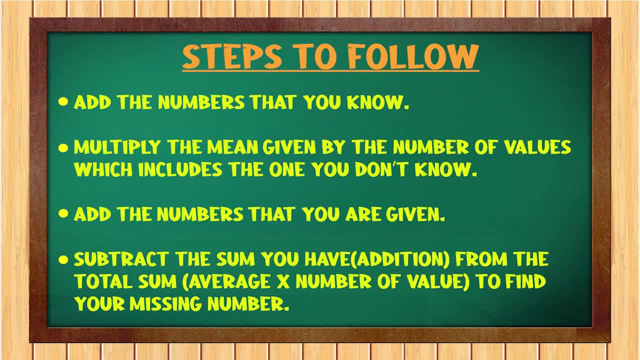 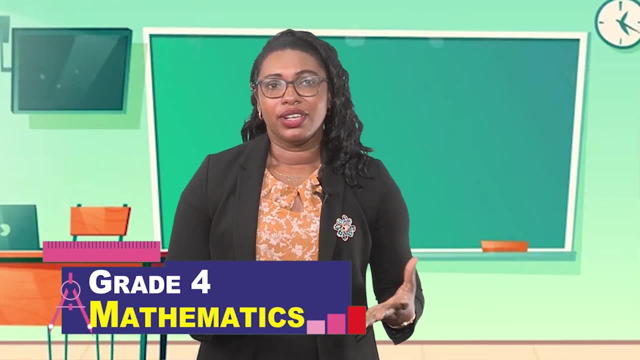 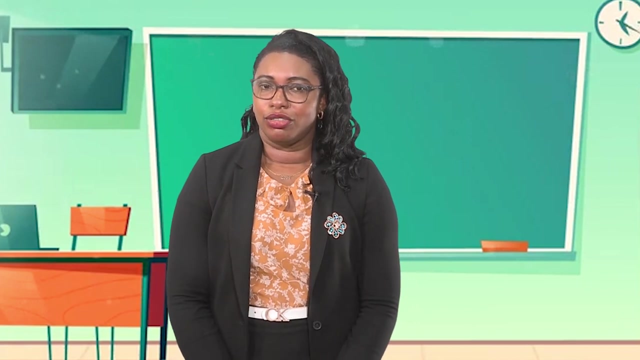 it and the total from the average multiplied by the number of values, to find your missing number. so the steps are pretty simple. you just have to keep practicing. and here again, I have for you homework. before we leave, so take a few seconds and write this homework down so that you could do it.